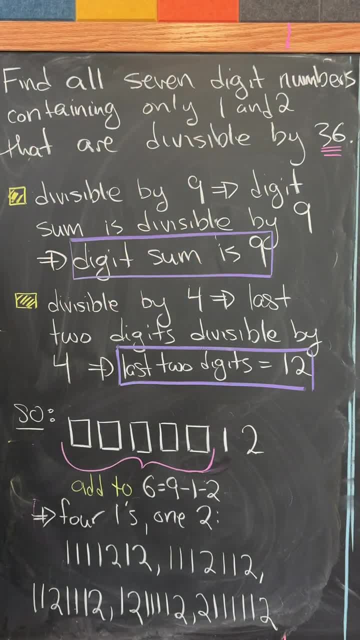 Let's find all of the seven digit numbers that only contain ones and twos that are divisible by 36.. Now, being divisible by 36 means you're divisible by nine and four. Being divisible by nine means the digit sum is divisible by nine, But with seven digits and only using ones and twos. 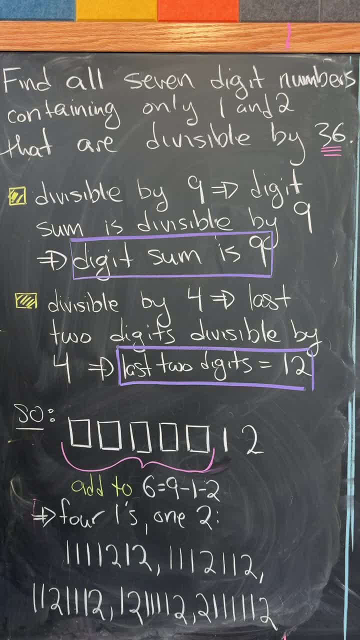 that means our digit sum is nine, Since a hundred is divisible by four. being divisible by four means the last two digits are divisible by four. That means the last two digits have to be one, two. Generally, our number looks like well, something, something, something something. 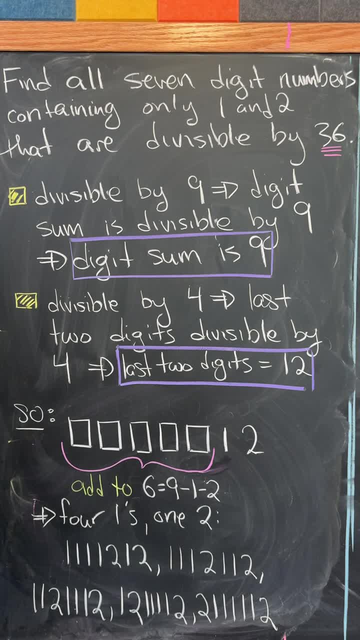 something, one, two. But then those five numbers at the beginning have to add up to six, which means we must have four ones and one two. Well, you've got five places to put that one- two. so there should be five total numbers. and here they are. 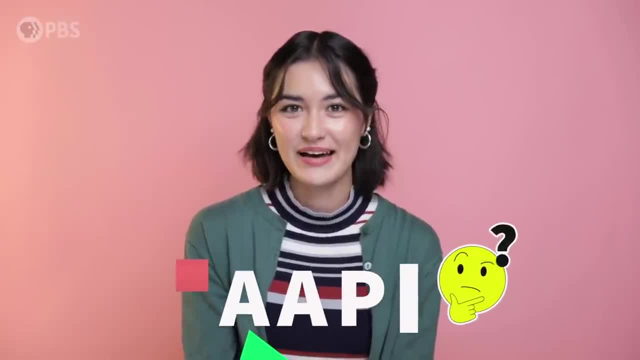 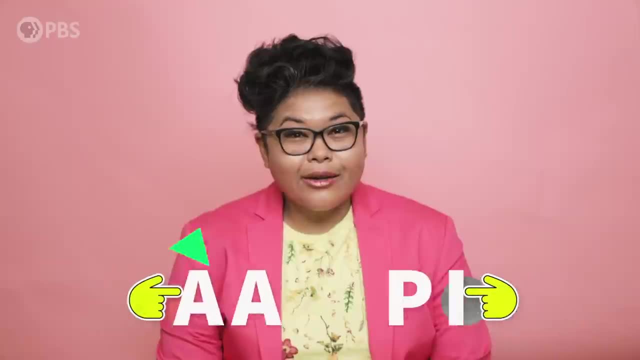 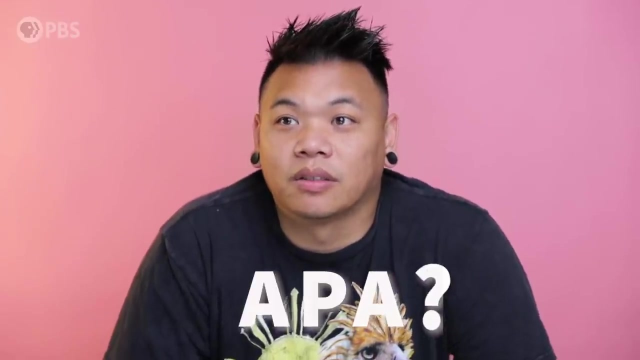 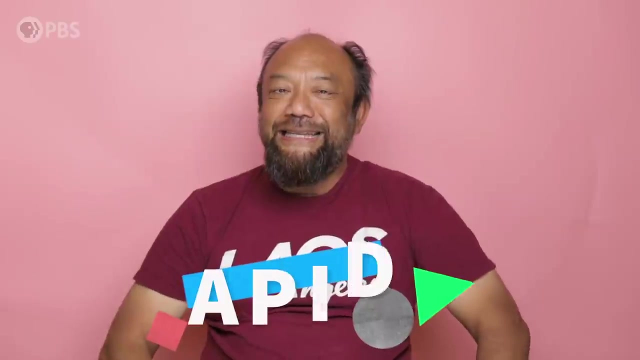 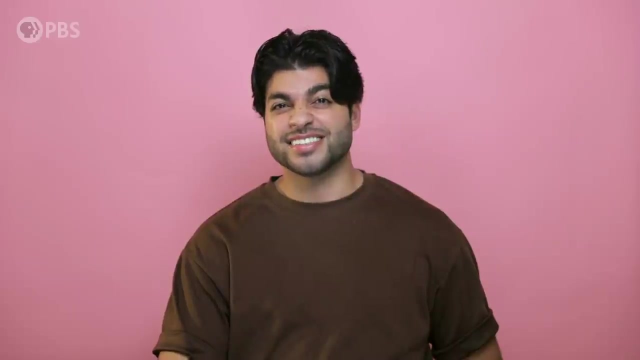 I think AAPI means Asian American Pacific Islander. Is that right? The terms AA and PI got lumped together because of the government, But it's officially APA, right? Who knows? Asian Pacific American, which makes no sense. Ooh, A-P-I-D-A. Okay. Asian Pacific American Indigenous. 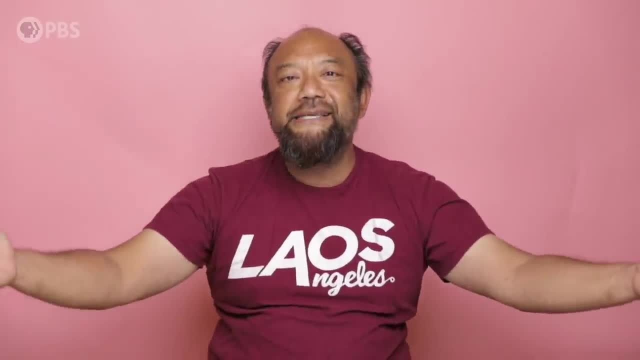 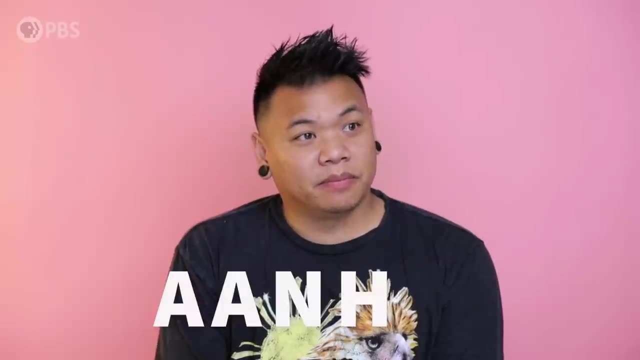 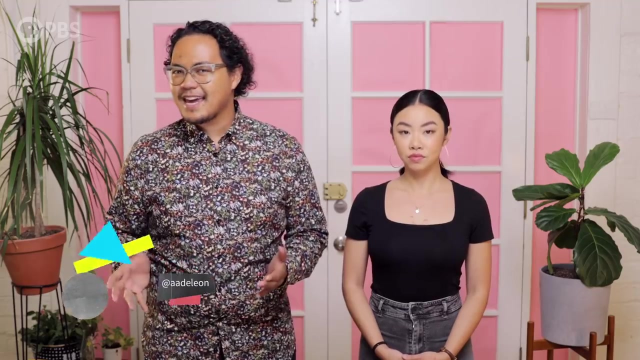 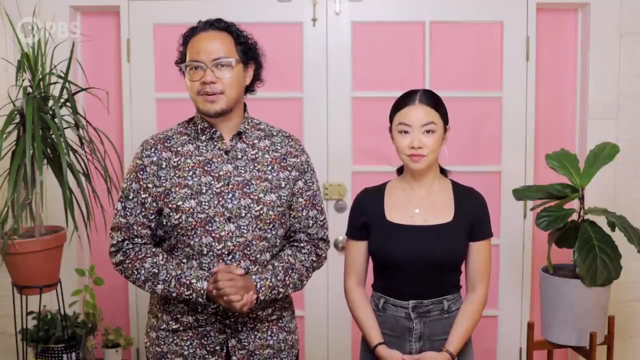 Asian Pacific Islander. Oh, Desi-American. Yes, yes, yes. Asian American Native Hawaiian Pacific Islander. Yes, Come on, It is AA NA H-P-I Heritage Month, officially declared so by President Biden just in time for May 2021.. 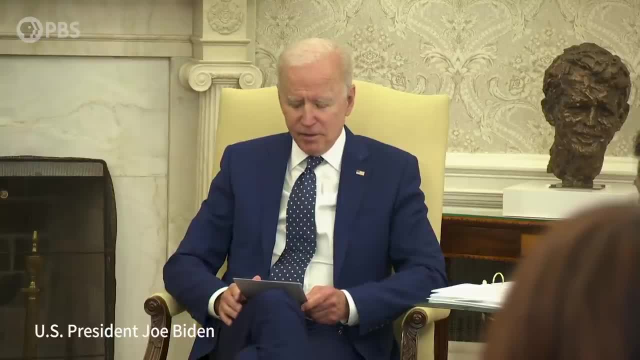 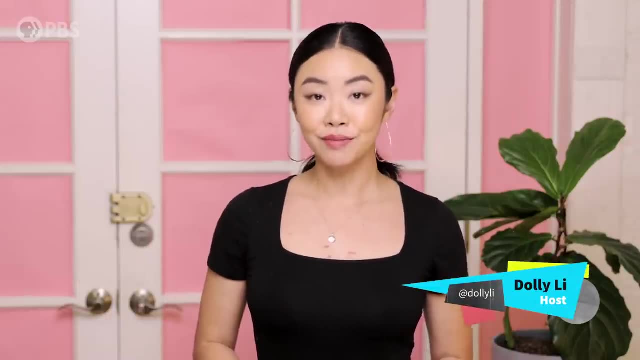 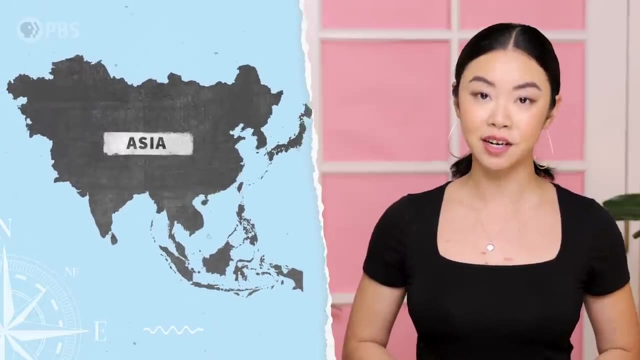 Vital communities and very diverse communities within the Asian, American, Hawaiian- excuse me- and Native Hawaiian and Pacific Islanders. Yes, it is a mouthful and includes a huge range of people who can trace their ancestry to one giant continent of over 40 different countries And about 25,000 islands in the Pacific Ocean.